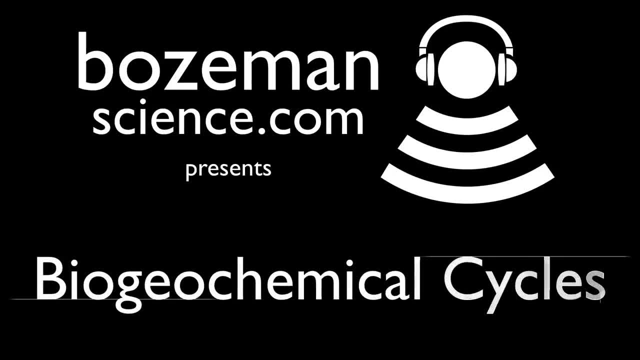 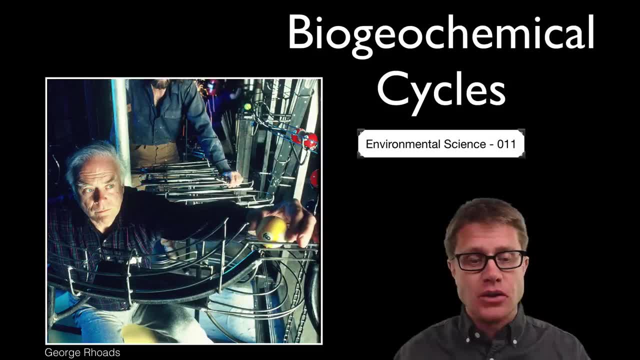 Hi, It's Mr Andersen, and this is environmental science, video 11. It is on biogeochemical cycles. This is a picture of George Rose. You have probably never seen him before, but you may have seen his work If you have ever seen a giant kinetic sculpture at a museum, where 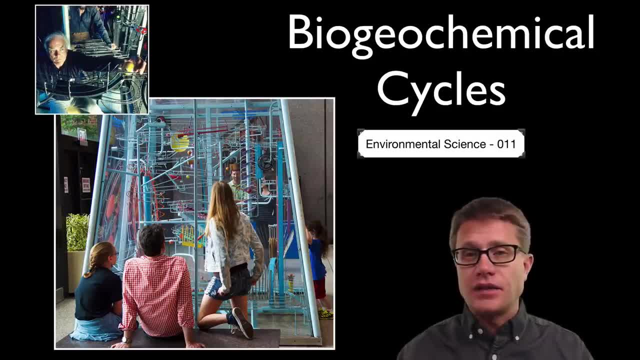 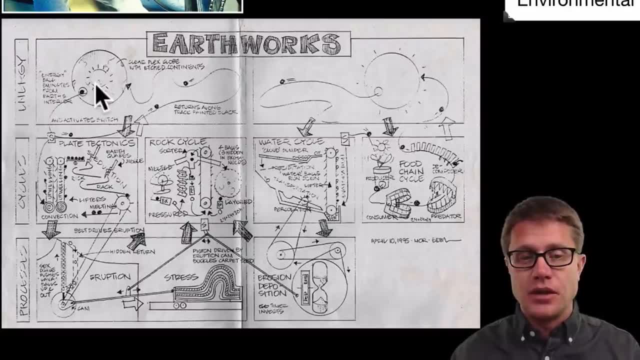 billiard balls are lifted up and then they move down again. he invented that and has installed lots of those around the world. Here is a planning document. In this one he is trying to show how energy from the sun or within the earth can drive things like. 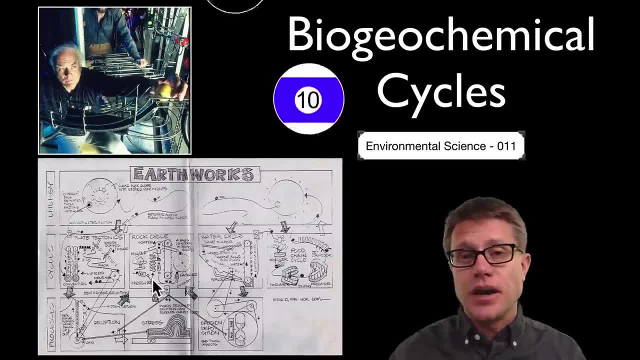 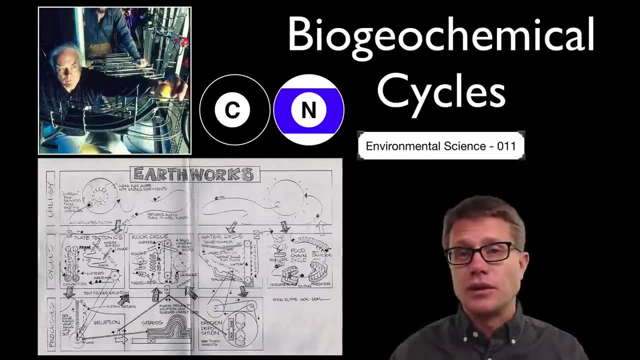 the water cycle and the rock cycle, And it is a really good model for how nutrients move around on our planet. The carbon and the nitrogen that we have is set and it just moves around between the living and non-living world, And so the matter on our planet is. 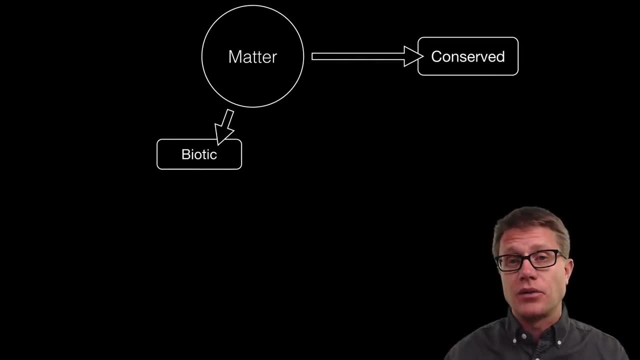 conserved. We have a set amount, and it moves between the biotic, or living, and abiotic world. The living world is called the biosphere on our planet, And the nutrients that we need are best remembered in this mnemonic schnapps: Carbon, hydrogen, nitrogen, oxygen, phosphorus. 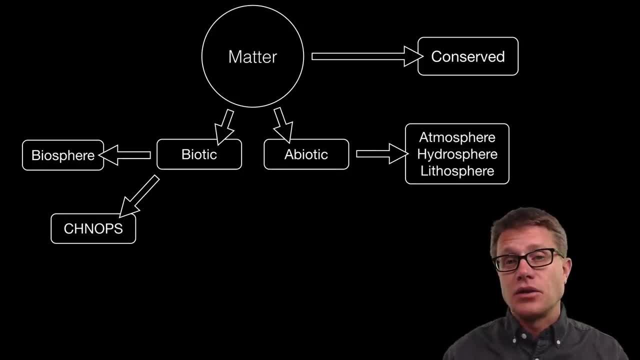 and sulfur. If we look at the abiotic factors, that is going to be the atmosphere, lithosphere and hydrosphere, And so these biogeochemical cycles is going to be how the nutrients move between the living and non-living. Now, why is it such a long word: Bio, geo and chemical? 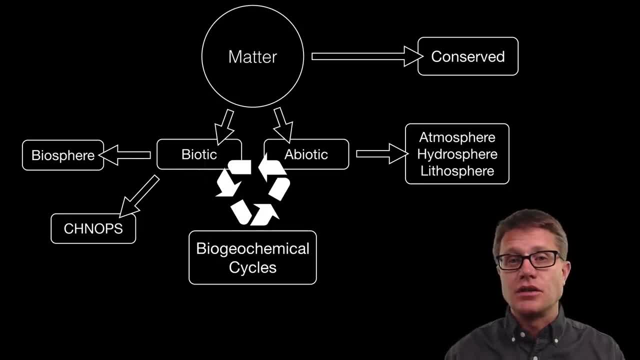 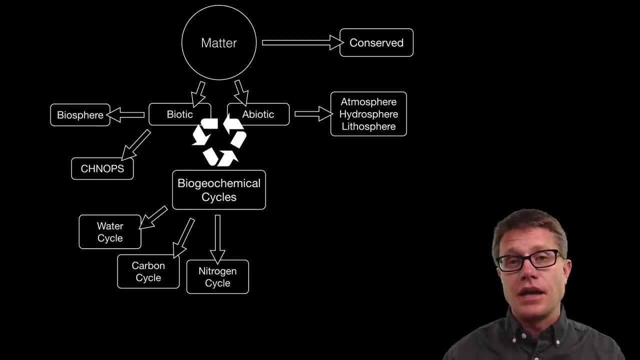 are the biological, chemical and geological processes by which the nutrients move around. You are probably most familiar with the water cycle. We will start there and then talk about the carbon cycle and, following that, the nitrogen cycle. One thing you are probably not familiar with with the nitrogen cycle is the importance of bacteria and how they can nitrogen fix. 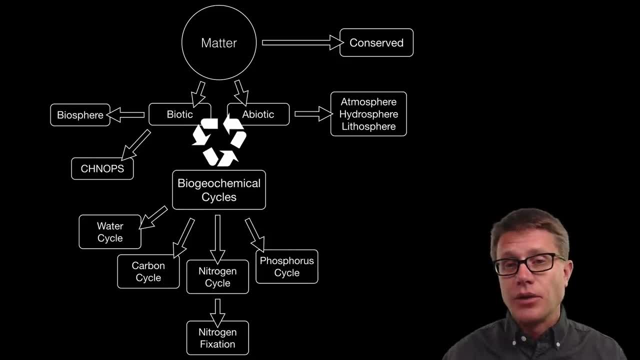 or take nitrogen out of the atmosphere and put it into the living world. We will then move to the phosphorus, one of the lowest, the slowest turning cycles. It involves rock, but no atmosphere. Now both nitrogen and phosphorus are what are called limiting nutrients. That 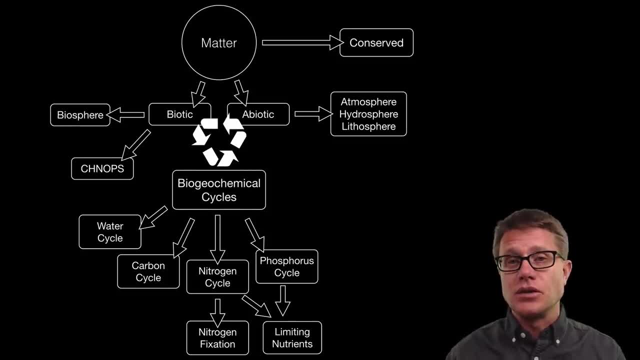 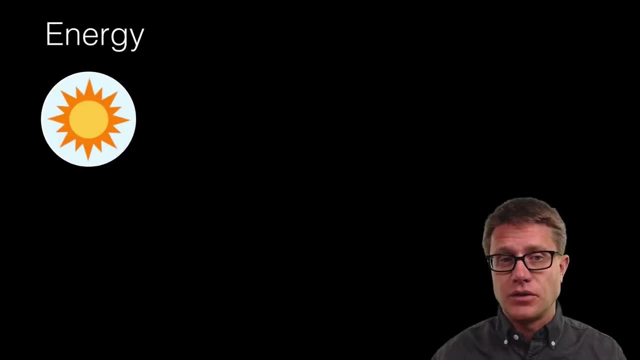 means life really needs them and it is waiting for them. And once it gets those nutrients, then it grows really, really quickly. That is a good thing, but sometimes can lead to eutrophication, And then finally, we will finish with the sulfur cycle, And so the 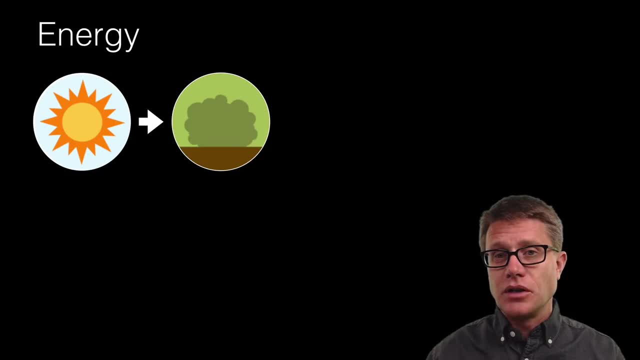 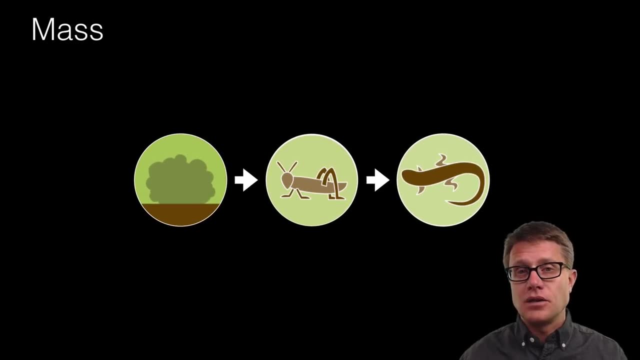 energy on our planet, remember, starts in the sun, moves through producers to consumers, other consumers, and eventually is lost as heat. But as we move to matter, everything on the planet is conserved. There is no sun anymore, And so how do the producers get the? 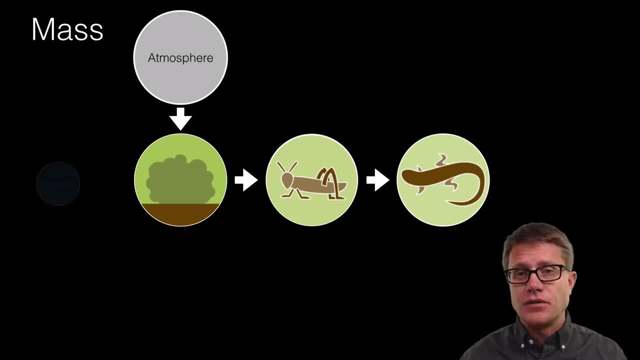 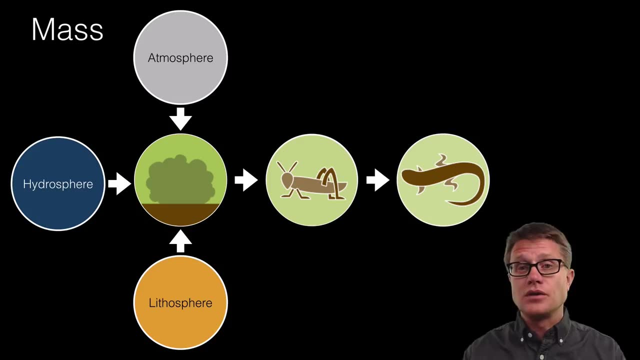 nutrients that they need. It is from their environment, From the atmosphere, from the hydrosphere, from the lithosphere. How do consumers get the matter they need? By eating plants, or eating consumers that ate plants? How does the matter go back into the environment? 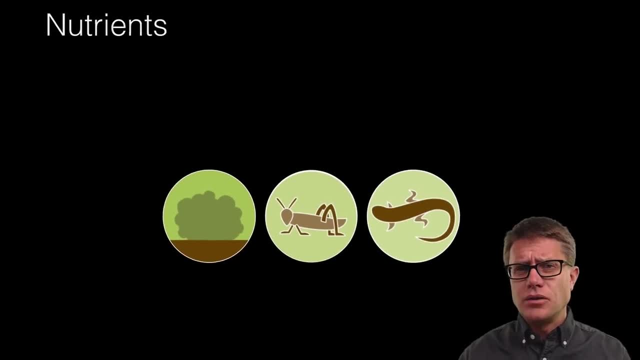 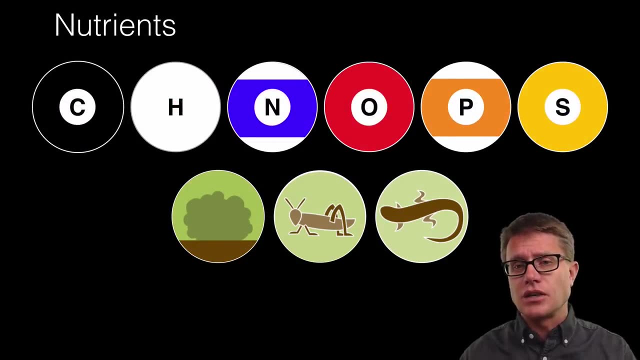 again Through these biogeochemical processes. So we are going to talk about the biogeochemical cycles, And so what are the nutrients that life needs? What are the billiard balls of life? Well, a good mnemonic is schnapps: Carbon hydrogen, nitrogen, oxygen, phosphorus and 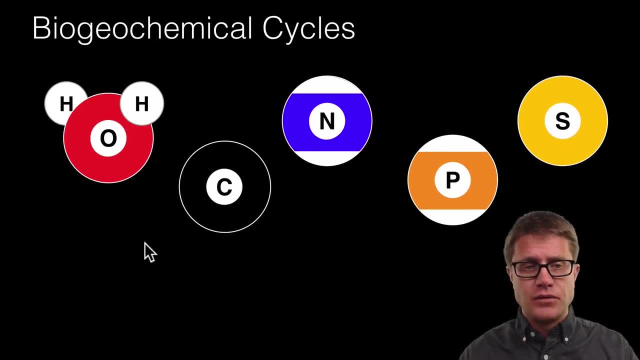 sulfur. If we organize that into the five cycles, we have got the water cycle, carbon cycle, nitrogen cycle, phosphorus cycle and sulfur cycle. So why do we need all of this matter? We are filled with water. We also use the oxygen to release energy and transfer. 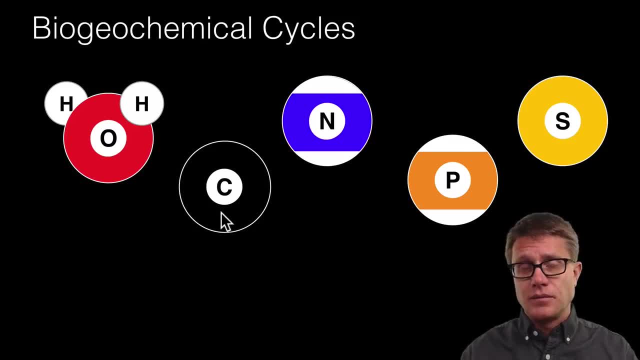 energy with the hydrogen. We are built out of macromolecules. That is what macromolecules. carbon is the building block of. The nitrogen and the sulfur are both big components in the proteins that make us up, And then the phosphorus is found in DNA, RNA and the ATP. 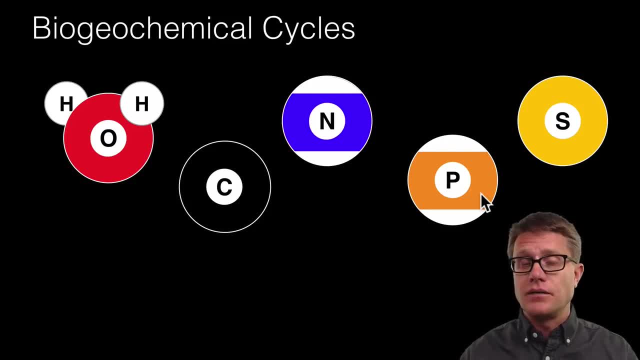 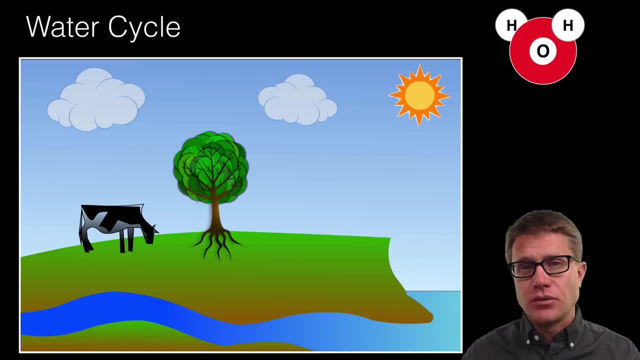 And so if we do not have these nutrients, if we do not have these atoms, then life cannot exist. So we need to pull them out of our environment. So let's start with the water cycle. How do plants get water? They are going to take it in through their roots. What about? 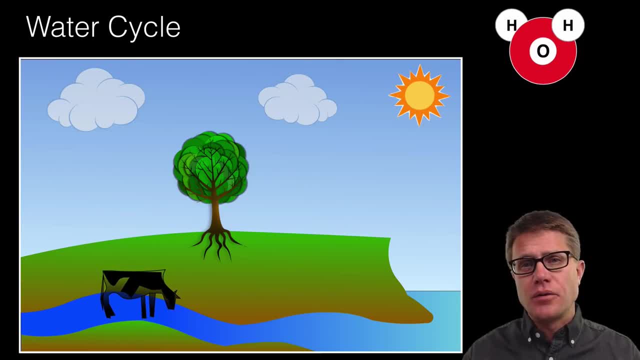 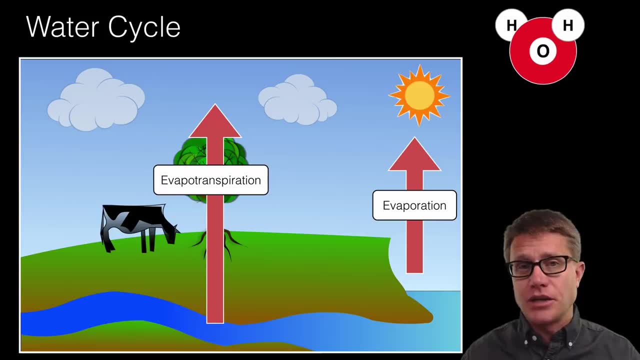 a cow. They are simply going to drink the water. But how does it move through the abiotic parts of our planet? First of all, we are going to have evaporation. We are going to have evaporation off ocean lakes and streams, And then we are going to have evapotranspiration. 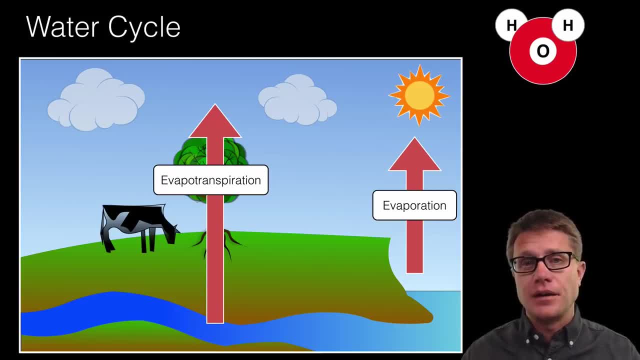 So it is evaporating, But also it is being transpired through the leaves of a plant. It is now moving from a liquid to a gas. What eventually happens is we are going to have condensation in the clouds, We have precipitation And then we have runoff over the surface and 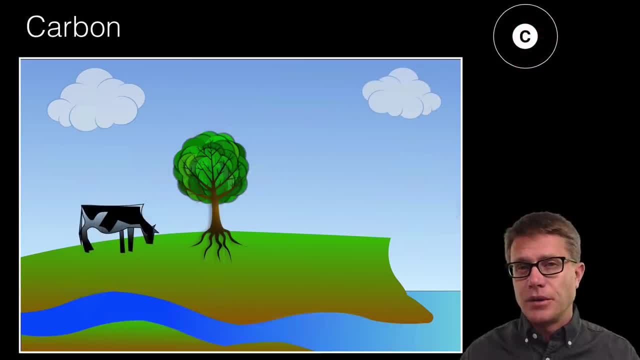 through ground water And the whole thing begins again If we start with carbon. how does a plant get carbon? It is going to be through photosynthesis, Both in plants on land and then phytoplankton that are going to be found in the ocean. What about an energy? 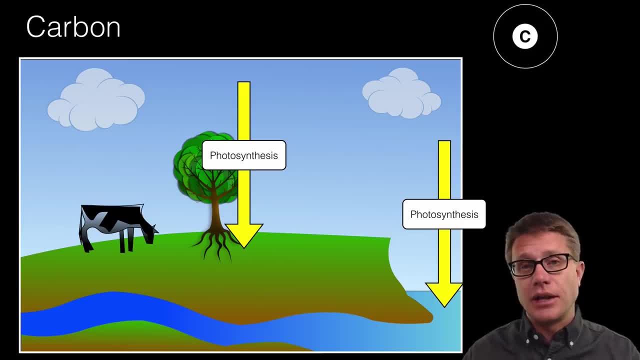 animal like this cow. It simply gets the carbon through its diet. It eats the plant, Or if something eats a cow like you, you are taking the carbon from the meat of the cow. So what happens to that carbon? It is eventually released through cellular respiration. It. 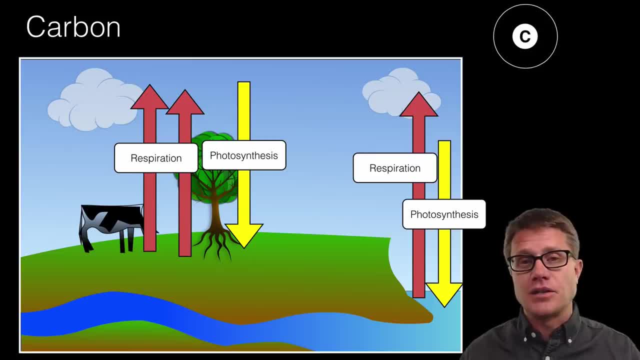 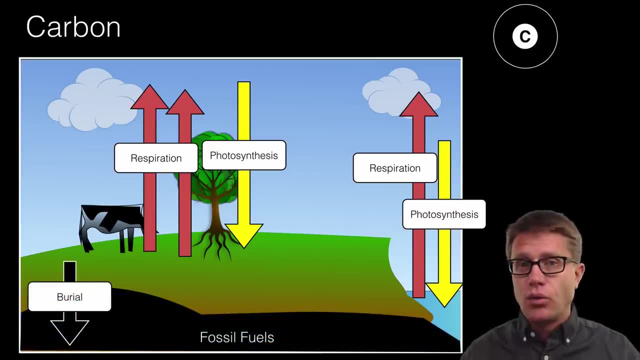 goes back into the atmosphere again as carbon dioxide. So a lot of that carbon is going to be in the atmosphere as carbon dioxide. Now we can also take that carbon and it can be covered by rock and we can create coal and oil fossil fuels. So we are storing that. 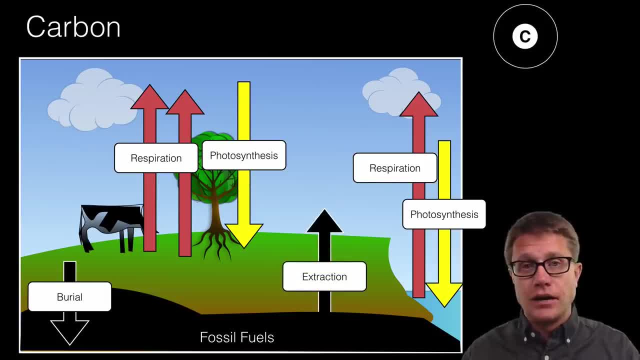 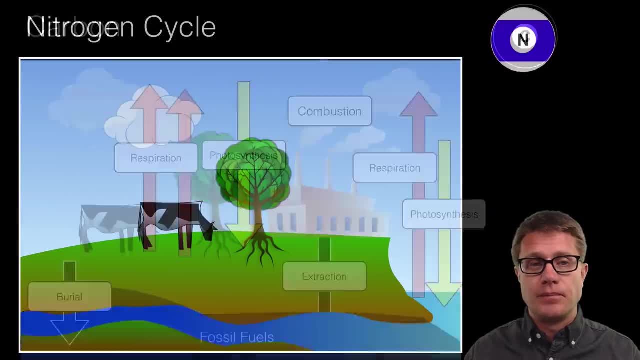 carbon in the rock. We can extract it again by digging a well And then we can have combustion, where a factory releases that carbon dioxide back into the atmosphere, And the whole cycle continues again. The nitrogen cycle is a little different. Most of the nitrogen is going to be found in the atmosphere as nitrogen gas. 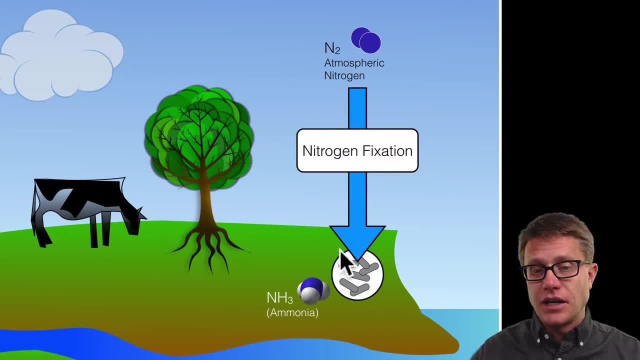 And to get it into the living systems we have to do nitrogen fixation. So there are bacteria that live lots of times on the roots of plants in these nodules And they are converting the nitrogen in the atmosphere into usable ammonia. We can also put ammonia on our fields. 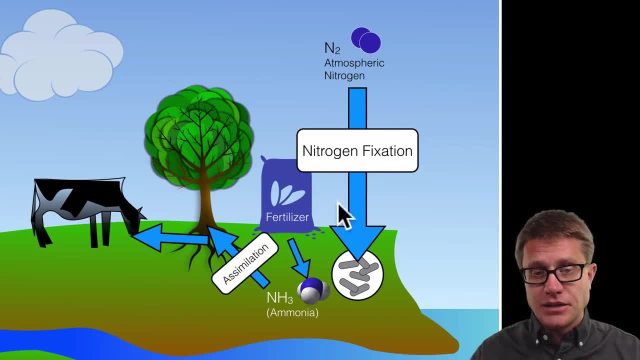 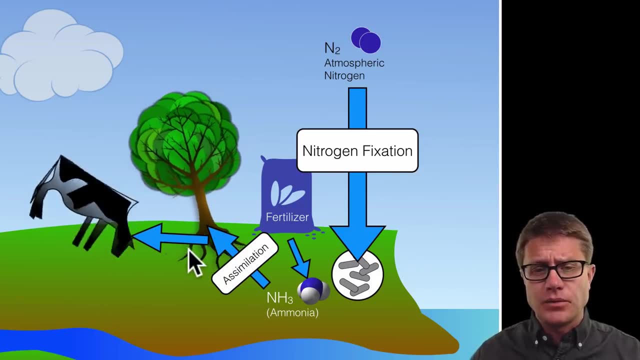 as fertilizer, And then it is going to be assimilated. In other words, plants are going to take it in through their roots and we are going to get it from plants simply by eating them. Now, how does it get returned back to the atmosphere? It is kind of complex. What happens is we. 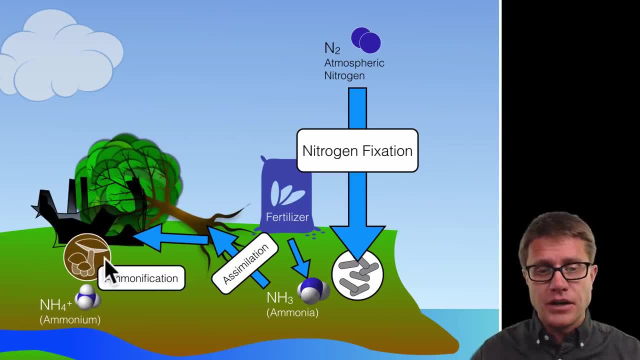 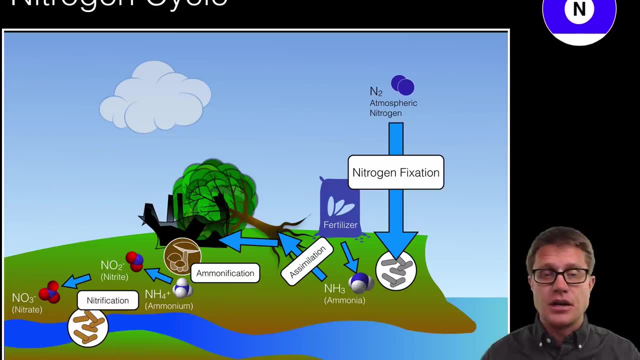 have death. We then have decay, And so bacteria or fungi are going to convert that nitrogen into ammonium. And then we have other bacteria, nitrifying bacteria, that are going to convert that ammonium into nitrites and then nitrates. Now the nitrates can be leached, They can 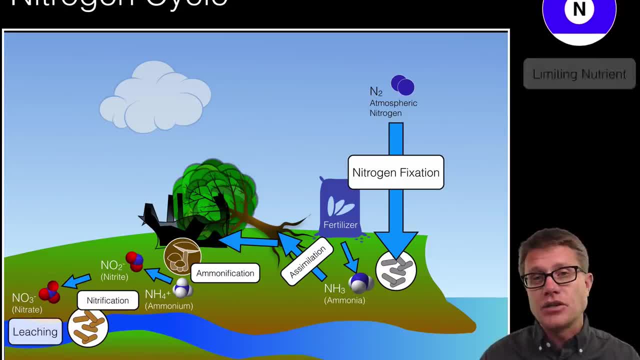 move into the water supply of our planet. Remember, nitrogen is a limiting nutrient. Plants, life is just waiting for nitrogen to be there And once we get nitrogen, for example in this stream, you will get an algae bloom, We will get a bunch. 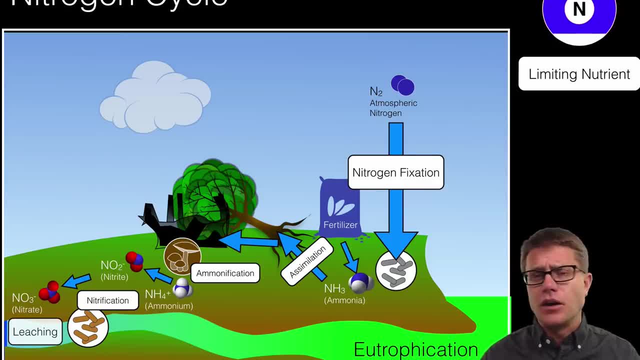 of algae growing really, really quickly. Now, that seems like a good thing, But all those algae are going to quickly die, And eutrophication is this process by which they die and then other bacteria have to break them down through respiration, And it consumes all of the oxygen. 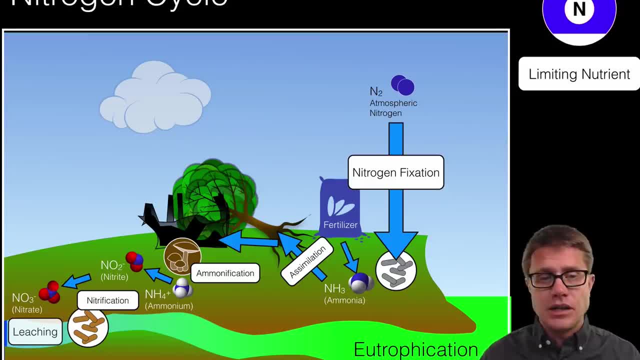 So it is not healthy for that water supply. But let's keep watching the nitrogen. How does he get back into the atmosphere? Well, the nitrogen is going to get back into the atmosphere. We will have denitrifying bacteria that are going to return it back into the. 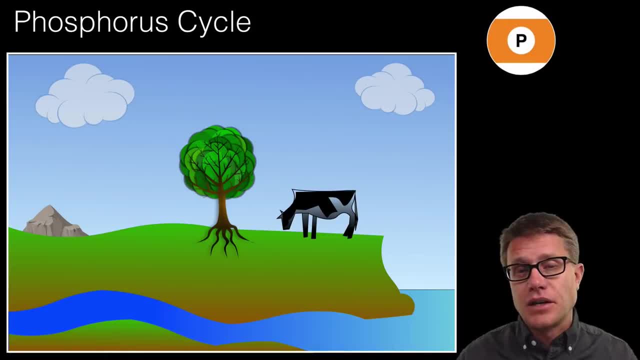 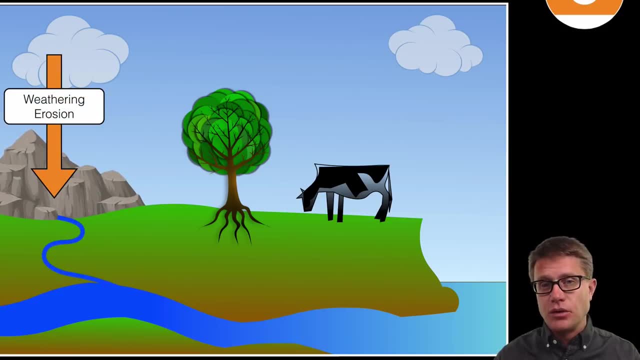 atmosphere, And so the whole thing can begin again. Now the phosphorus cycle is going to turn more slowly. It starts by having rock that have phosphorus being uplifted. We then have weathering and erosion, And that is going to move the phosphorus into the soil, into 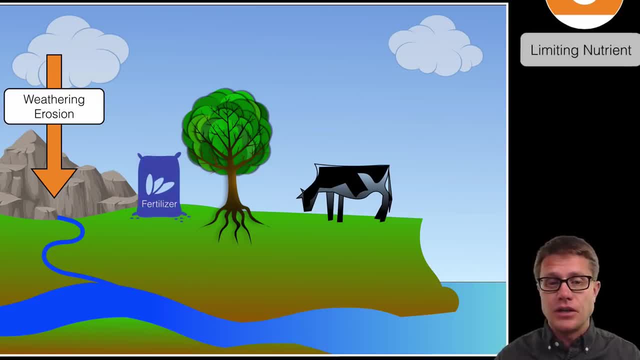 the water supply. We could also add fertilizers. That is going to have phosphorus, And the whole thing, since it is limiting, can promote eutrophication. What happens to the phosphorus? We then have assimilation, where it is taken into plants. We can eat the plants and we 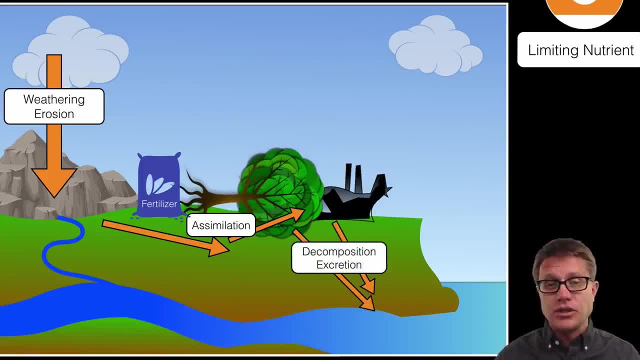 get it. What eventually happens is we die. So, through excretion and decay, we return that phosphorus into the water supply. It eventually works its way to the ocean, And then it eventually settles out in these sediments, And so it never goes to the atmosphere. It. 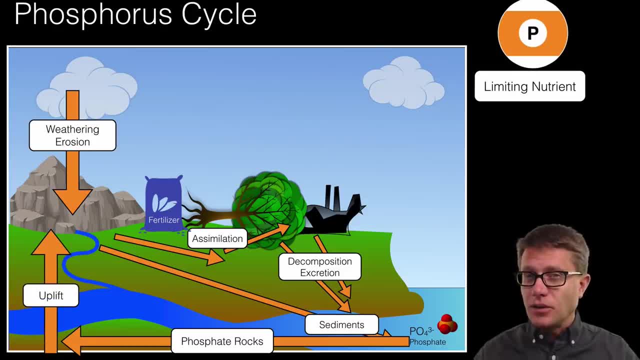 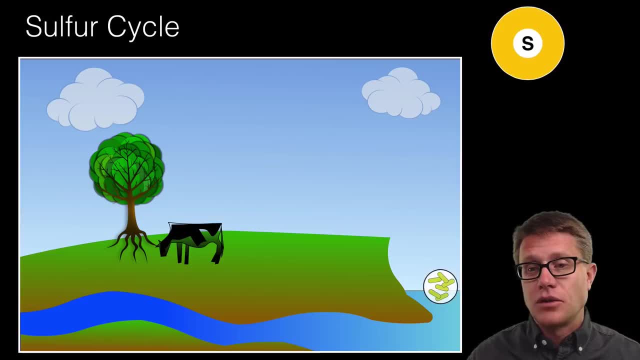 becomes part of these phosphate rocks, which are then uplifted again, And so it takes a long time for this cycle to turn, because we do not include the atmosphere, And then, finally, we have the sulfur cycle. Sulfur cycle is going to move from the oceans, the sulfur. 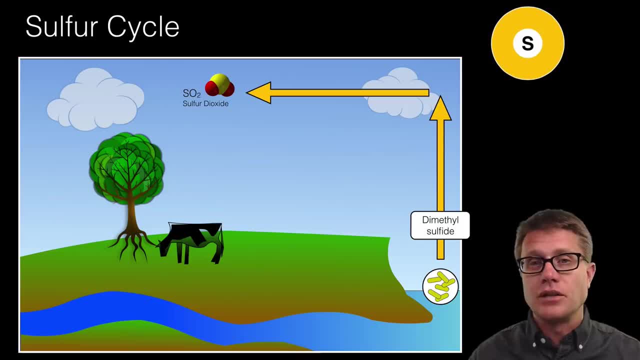 we have bacteria that are going to convert that into dimethyl sulfan fans because nano dimethyl sulfide, which eventually becomes sulfur oxide or sulfur dioxide. We can also increase sulfur dioxide through volcanism, So volcanoes are releasing hydrogen sulfide, which becomes sulfur dioxide, And then factories are going to release sulfur dioxide as well. 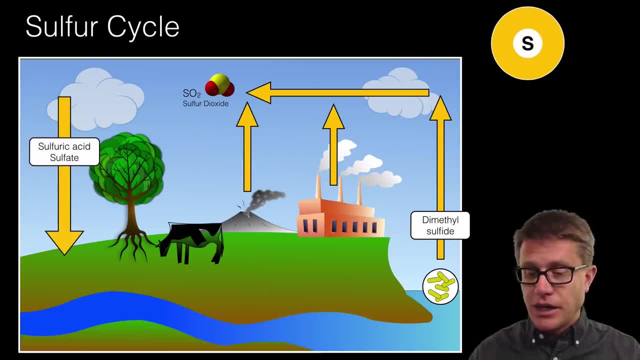 It is in the atmosphere. now How does it get back to the planet? It is going to rain down as sulfuric acid and sulfates. We can then assimilate that, Take it into the living material, same way Into plants and then into consumers And finally it works its way back through. 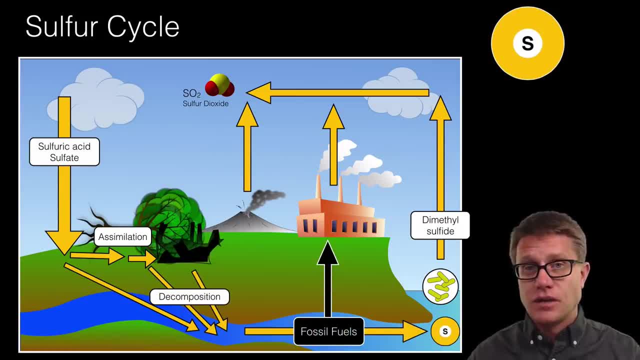 the water supply, and now it is going to be sulfur in the oceans. So the cycle could continue again. But we can also have that rock cycle forming some of that into fossil fuels which can be extracted again, and the cycle continues. And so for each of these cycles you should 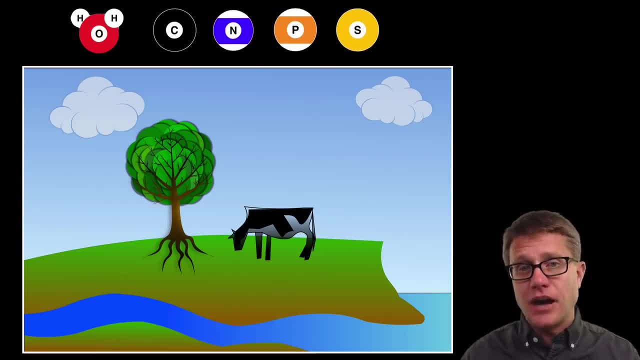 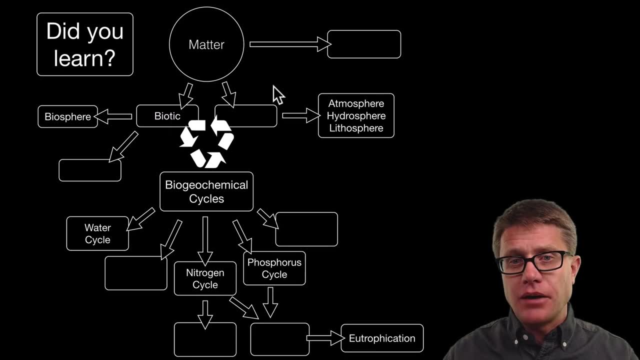 be able to figure out how do plants get it, How do animals get it, And then how does it recycle back through the atmosphere, hydrosphere and lithosphere. So did you learn the following? Could you pause the video right now and fill in the blanks? Remember, matter is conserved. 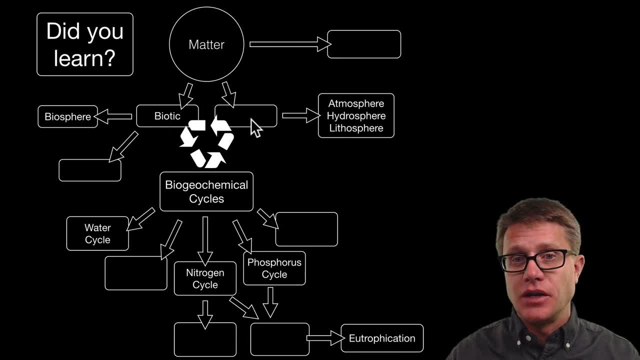 on our planet. We have a lot of matter on our planet. We have a lot of water on our planet. We have a set amount. It moves through the biotic and abiotic spheres. A good way to remember the nutrients we need is schnapps. The biogeochemical cycles are how we move. 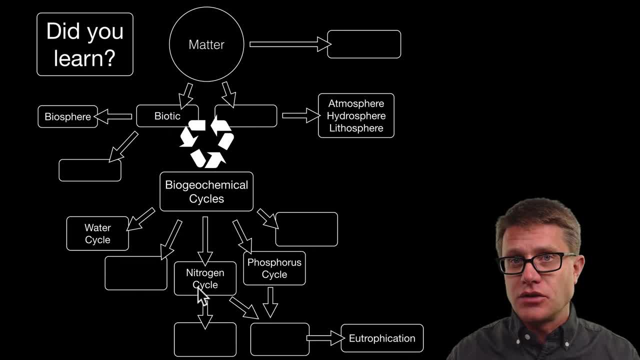 it through abiotic and biotic. It is the water cycle, carbon cycle, nitrogen cycle which requires nitrogen fixation. Remember, nitrogen and phosphorus are limiting nutrients which can lead to eutrophication. The last cycle is the sulfur cycle And I hope that was helpful. Thank you very much.